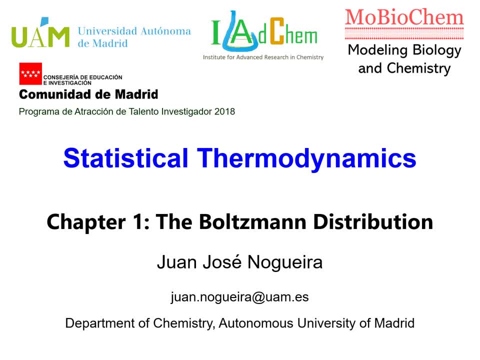 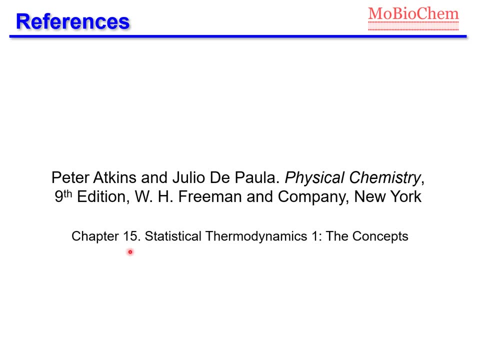 Welcome to a new lecture by the MobioChem research group. We are going to start a new series of lectures about statistical thermodynamics and in particular, today we are going to talk about the Boltzmann distribution. This lecture is based on the chapter number 15, Statistical Thermodynamics, from the book by Peter Atkins and Julio de Paula, Physical Chemistry. 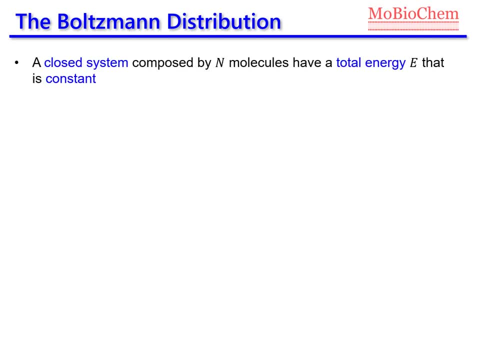 Okay, so let's start. Let's assume we have a system, a closed system, which is composed by M molecules, and the system has a total energy, E, which is constant. In addition, the collisions between the different molecules which compose the system will induce a redistribution of the total energy between the molecules and also between the different modes of motion. 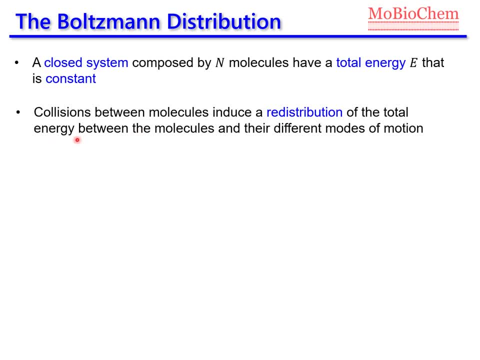 However, as I said before, the total energy of the system is constant. So our goal is to determine how many molecules and I occupy a particular state with energy EI, Because if we know the distribution of our molecules among the different states, then we can compute the properties of this particular system. 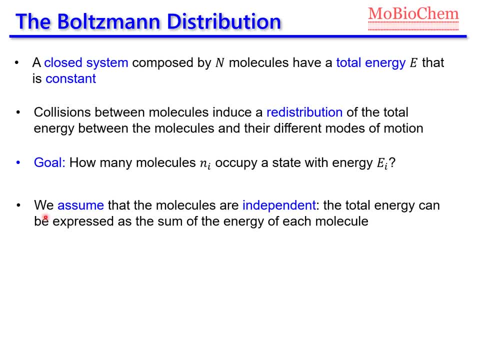 So we are going to assume that the molecules are independent. That means the total energy can be written as a constant. So the total energy can be written as the sum of the energy of each individual molecule in the following way: So that means we are neglecting the intermolecular interactions. 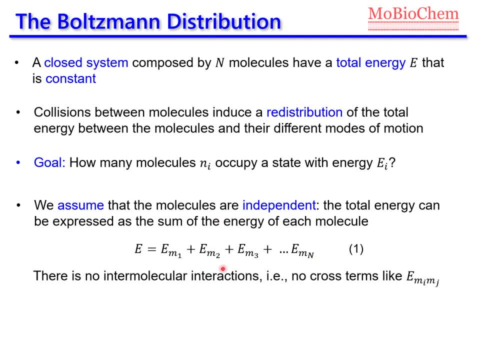 Or in other words, in equation number 1, we don't have cross terms like this one. So, for example, we don't have a term which provides the interaction energy between a particular molecule I and a particular molecule K, So we only have the sum of the energies of each particular molecule in this particular state. 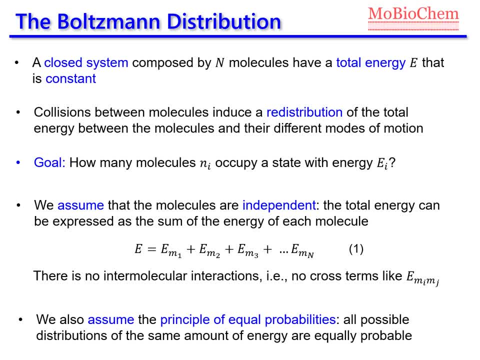 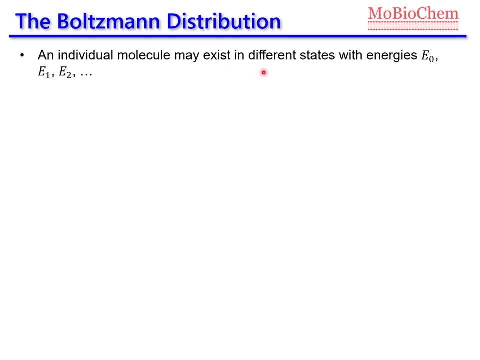 In addition, we are going to assume also that the principle of equal probabilities, That means that all possible distributions of the same amount of energy are equally probable. So an individual molecule may exist in different states with energies, for example E0, E1, E2, E3, and so on. 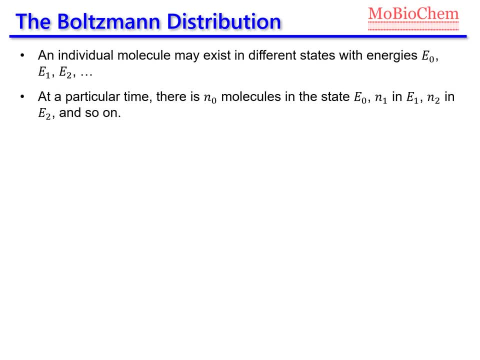 So, for example, at a particular time we can have, for example, N0 molecules in the state with energy E0, N1 molecules in the state with energy E1, N2 molecules in the state with energy E2, and so on and so forth. 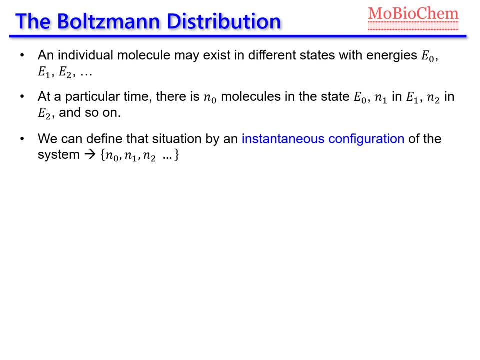 So, in other words, we can define a particular situation at a particular time by an instantaneous configuration where, for example here we can write in brackets the number of molecules that we have in each particular energetic state. For example, let's say we have four molecules and three states in our system. 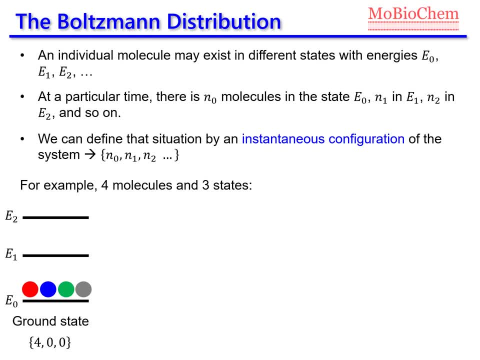 So this will be the ground state of our system, right? So we have the four molecules in the lowest energy level and this will be the instantaneous configuration. So four, zero, zero. So four molecules in the first state and then zero molecules in the second state. 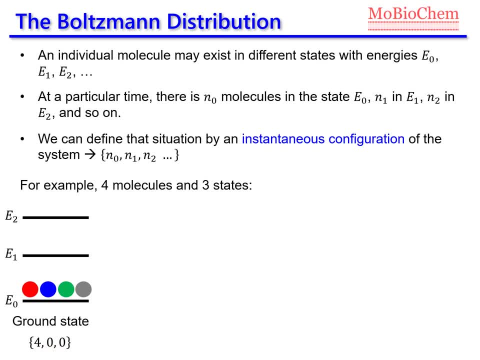 And then zero molecules in the other two remaining states. How is the first excited state of the system? So we can, for example, excite the red molecule to the E1 level, but we can also excite the other molecules, right? 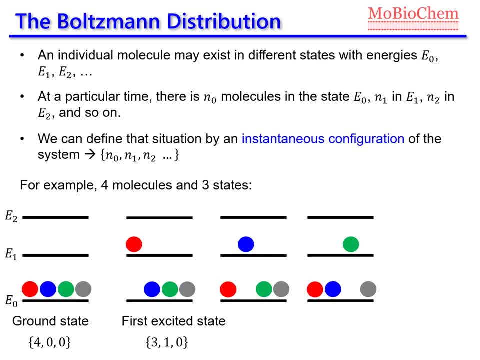 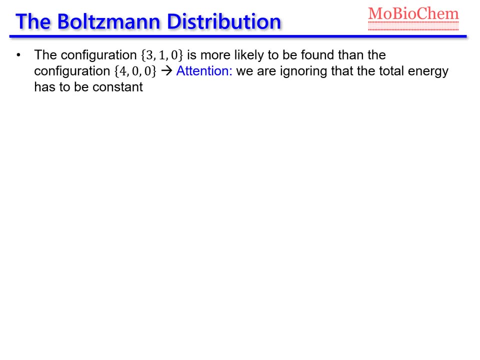 We can have the blue molecule in the E1 level. We can also have the green molecule or the gray molecule. So the configuration three one zero can be achieved in four different ways, As we can see here in the picture. So that means that the configuration three zero one is more likely to be found than the configuration four zero zero. 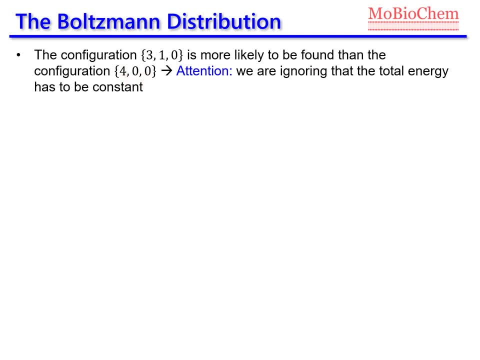 Why? Because, as we said, the configuration three- one zero- can be achieved in four different ways, while the configuration four- zero zero- can be achieved only in one way. Of course, we need to pay attention that we are in a system. 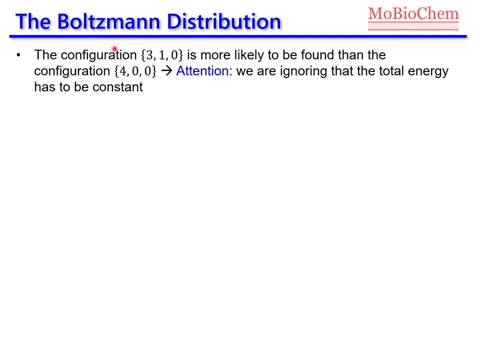 where we are ignoring the fact that the energy of these two configurations are not the same. So we are ignoring that the total energy has to be constant. But we are doing this for the sake of simplicity in this comparison because in reality, of course, the ground state probably is more likely to be populated, right. 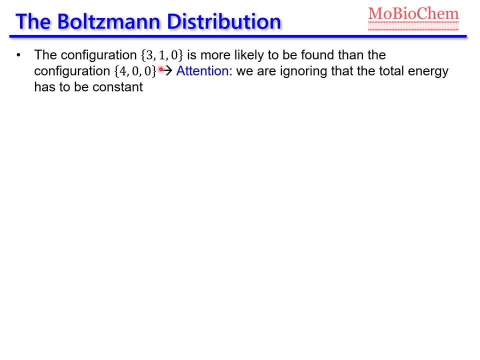 Because the energy is lower. But if we assume that these two configurations have the same energy, then the configuration three one zero is more likely to be populated right, Because the energy is lower, And the configuration three zero zero can be found. 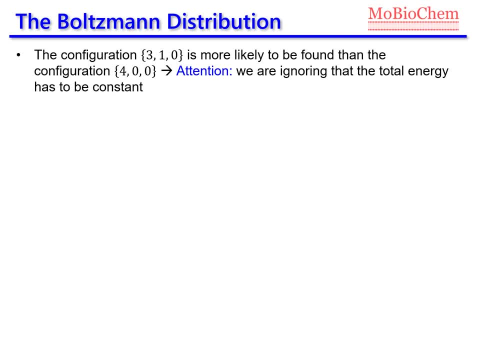 because, as we said, there are four different ways to achieve this configuration. So a particular configuration can be achieved in w different ways, where w is what we will call the weight of the configuration, And this weight of the configuration can be computed with equation number two. 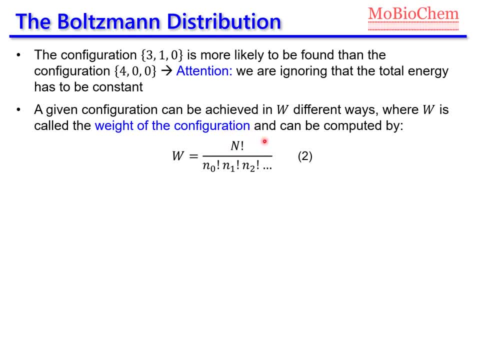 where we have here the factorial of the total number of molecules divided over the product of the factorial of the total number of molecules, the number of molecules in each particular state. So, for example, from the previous system, the ground state configuration, employing equation two: 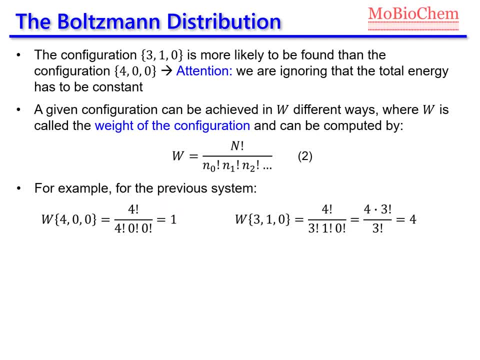 can be achieved only in one way. as we already said, However, the configuration three one zero can be achieved in four different ways. This is important because, for example, if the system oscillates between the ground state and the configuration three zero one. 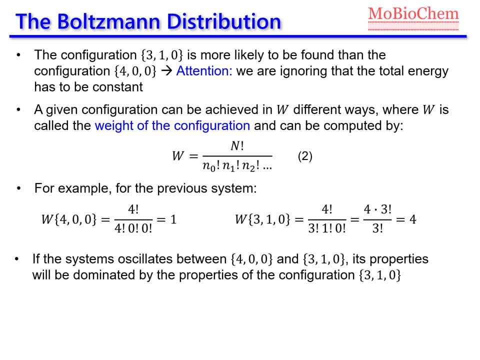 the properties of the system will be dominated by the properties of the configuration three zero one because, as we said, there are four different ways to achieve this configuration. or, in other words, the system will spend more time in the configuration three one zero and therefore the properties 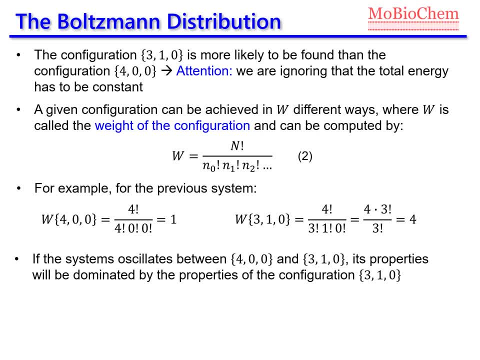 will be dominated by the properties of this particular configuration. Therefore, our goal is to find the energy configuration which has the largest weight, because this weight will determine the properties of the system. So let's now start working with equation number two. but we are going to work with the logarithm. 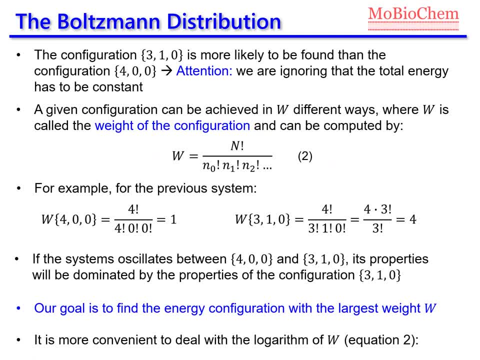 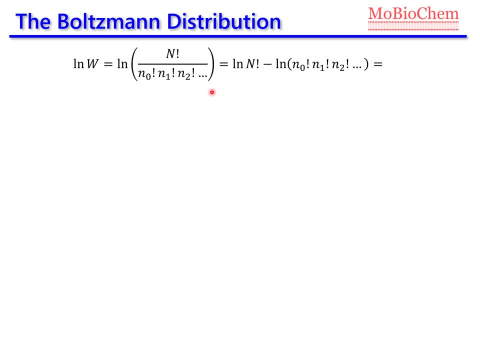 of this equation because, as we are going to see later, it will be more convenient. Okay, so here we have the logarithm of equation two, and now, when we go from here to here, we only develop this fraction, the logarithm of a fraction. 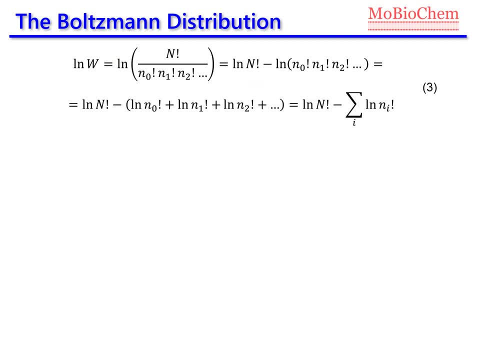 as the difference of these two logarithms. And then, in the next step, instead of having here the product of a logarithm, we have here the summation of different logarithms, And finally, in the last step, we group all these terms. 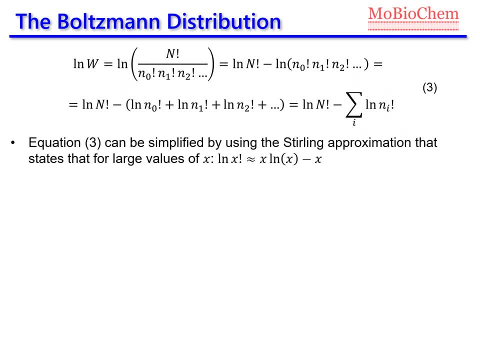 in just one summation. here We can simplify equation three by applying the Stirling approximation. that states that for large values of x the logarithm of the factorial of x can be simplified with this equation. So here we can assume that n is very large. 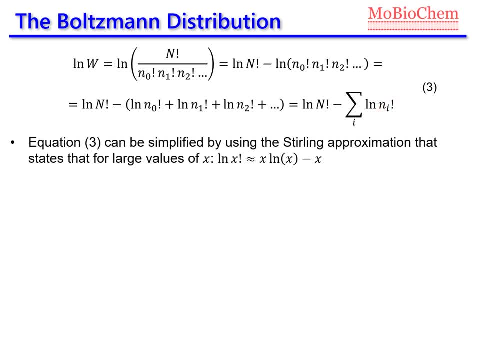 and also the number of molecules in each particular state will be very large because we are dealing with macroscopic systems. So, applying the Stirling approximation to equation three, We can write this equation here, where the logarithm of the factorial of the total number of molecules can be written in this way: after applying the Stirling approximation and the logarithm of the factorial of the number of molecules in each particular state, i can be also written in the same way here: 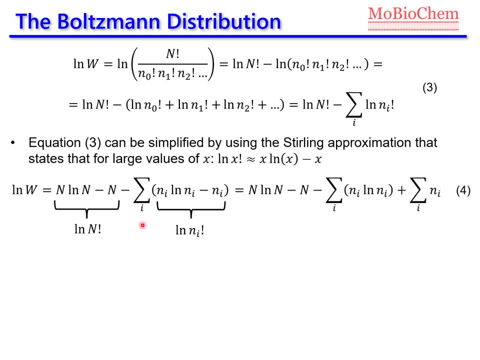 Now, in the next step, we can separate this summation in these two summations, here And now. this term is the summation of the number of molecules in each, in every particular state i, which is equal to the number of total molecules. 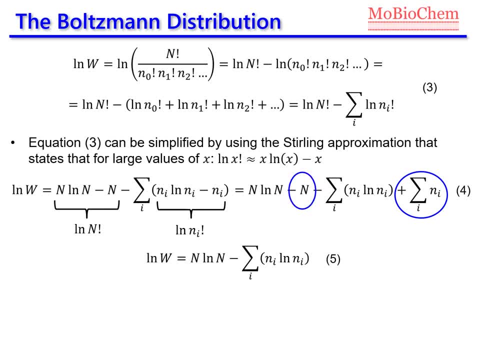 So this term here and this term cancel out and we can write the equation as equation 5 here. So, as we said, our goal is to find the configuration which has the largest weight right, Because this configuration will dominate the properties of the system. 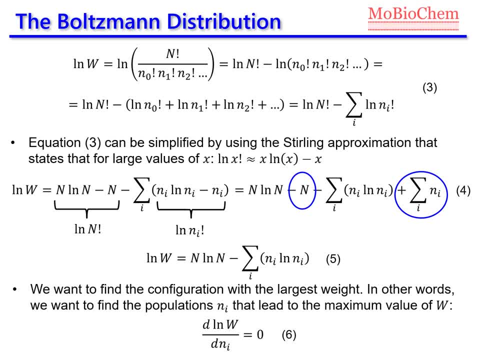 So, in other words, we want to find the populations in i that lead to the maximum value of w. So we need to do the derivative of this equation, number 5, with respect to the population of the states i. So doing this derivative, and doing this derivative equal to 0, we are going to find the maximum of this function. 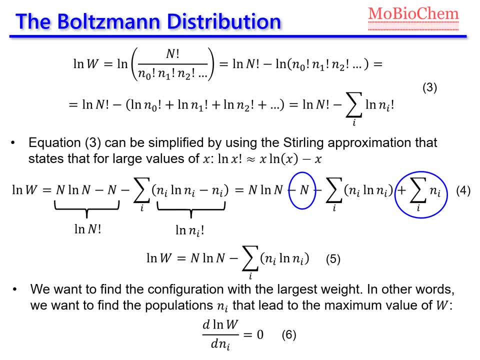 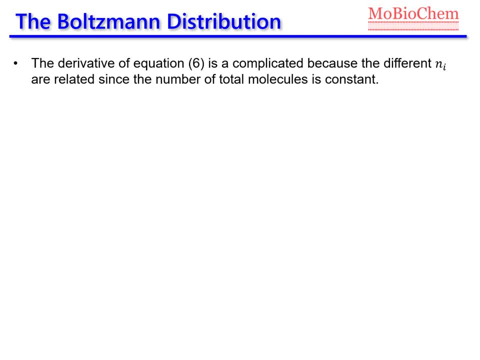 We are going to find the maximum of w. The derivative of equation 6 is a bit complicated because the different number of molecules in each particular state are related with each other because the total number of molecules is constant. For example, if the number of molecules in the state number 1 increase, then the number of molecules in other states has to decrease because the total number of molecules has to remain constant. 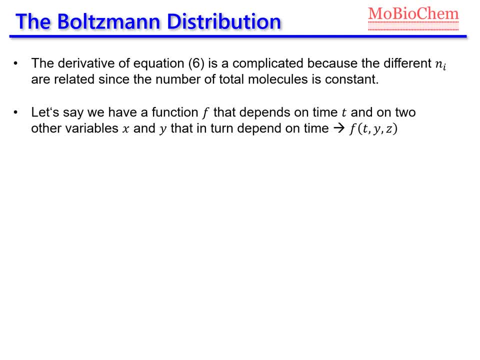 So that's it. That means, talking in general, that we have a function, f, that depends, for example, on a variable, let's say the time, And then we have other two variables, x and y, that in turn also depend on the time. 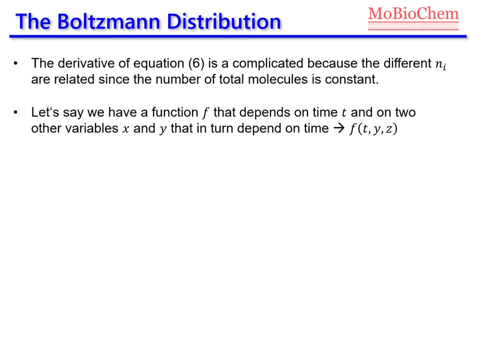 So we have variables which depend on each other. So when we want to compute the variation of the function with time, for example, what we need to do is the total derivative or the function derivative in order to introduce the dependency of x and y with the time, for example. So if we 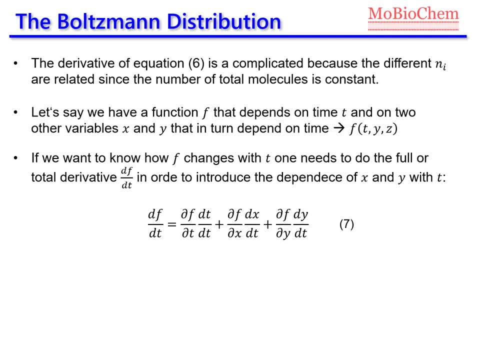 want to do the derivative of the function with respect to time. what we need to apply is equation number seven, where we have the partial derivative of the function with respect to time, the partial derivative of the function with respect to x and the partial derivative of the function with. 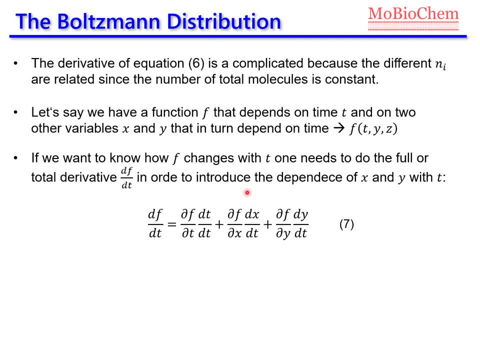 respect to y. and now we also need to multiply by the derivative of each of the variables with respect to time. so this is the definition of the total derivative, which can be written in the following way- just simplifying here this term, because this is equal to 1.. 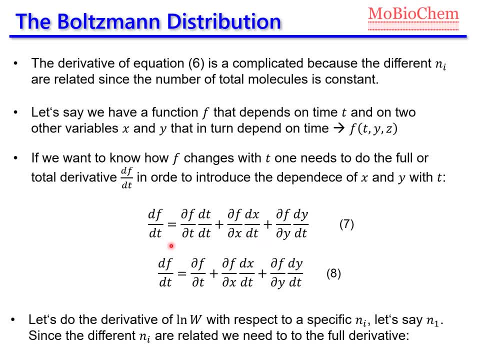 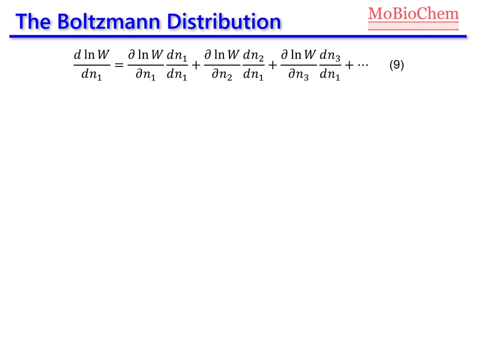 So let's apply the same rules. so let's apply equation number 8 to our particular system, so to the logarithm of w, because what we are going to do is to do the derivative of the logarithm of w with respect to a particular population. n i, for example, n1.. 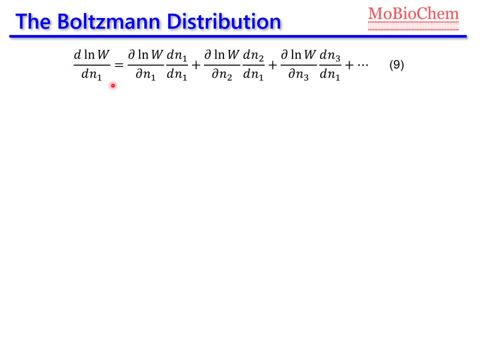 In. here we have the variation of the logarithm of w with respect to the population in the state number 1, using the definition of the total derivative. So this equation can be simplified In the following way: because this term here is equal to 1, and now we can multiply both. 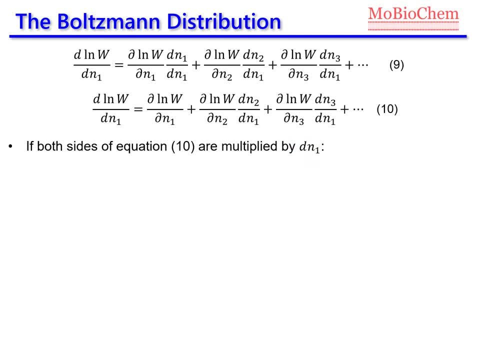 sides of equation 10 by the variation of the number of molecules in the state number 1, and we get the following equation, where the right-hand term can be grouped in one summation in the following way: So now we are going to modify this equation. we are going to modify equation 12 by n. 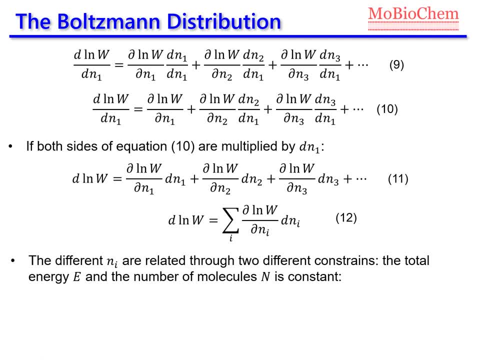 So we are going to multiply this equation 12 by n, and we have already made an exception of this whole declaration, and so we had the operation that we let to this term be a constant, of which the value of q at, we used as the parad Reverend. 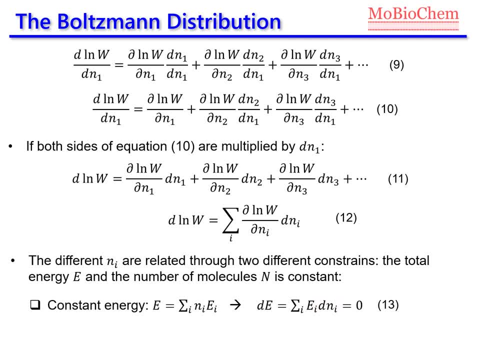 Now just randomization. we can even use the, as we talked about. Remember ein. we want clearünde a v at n, because this is a very significant property of the n-standard elephants In the following way: because this equation brings together the individually parametric. 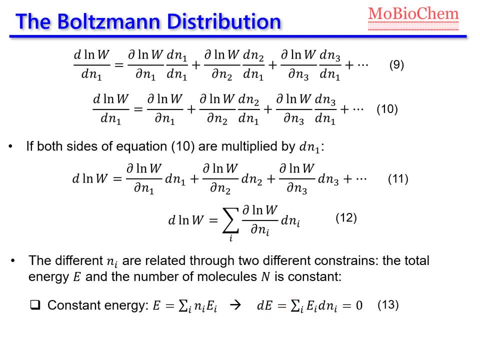 by the energy of each state, And this variation has to be zero. This is equation 13.. The second constraint is that the number of molecules, capital N, has to be constant, And the number of molecules is just the summation of the population of each particular state And the 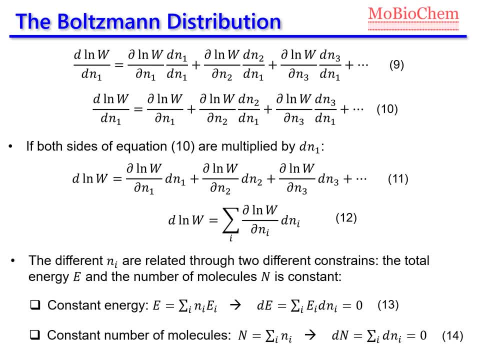 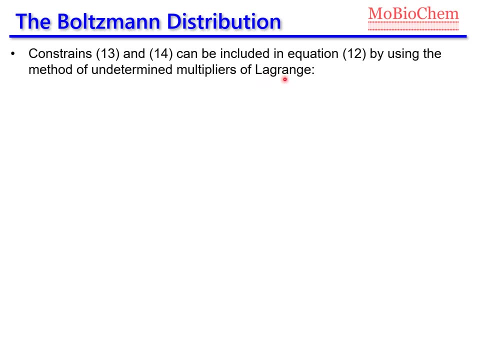 variation of the population, as we said, has to be zero. So these two are the constraints that we are going to introduce in equation 12.. And these constraints can be introduced by using the undetermined multipliers of Lagrange's method. So, after applying this method, equation 12 becomes: 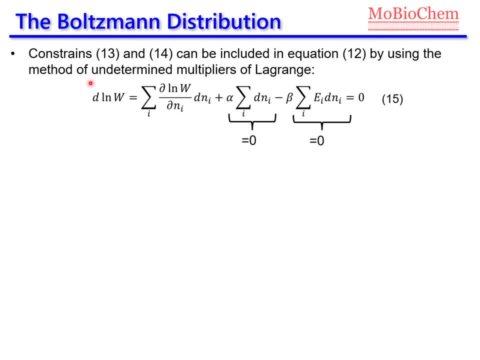 equation 15, where here? so this part of the equation is just equation 12.. And now we are here introducing our constraints, And here we are not doing anything illegal, because this term is equal to zero, as we see before, because the variation 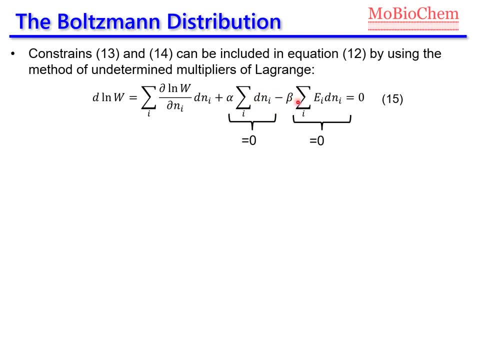 of the number of molecules has to be zero And also the variation of the total energy has to be zero. And these two constraints are multiplied by these two factors, alpha and beta, which are the Lagrange multipliers. Okay, so now we have the variation of the number of molecules in the state. 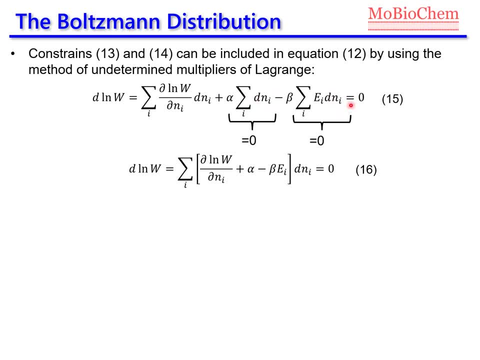 alpha and beta. And now we have the variation of the number of molecules in the state alpha and beta. Now we are multiplying the 시간. ничего enslaved molecules or the relation between these values are already included in the equation with the constraints. okay, So that means that we can assume that the variation of the 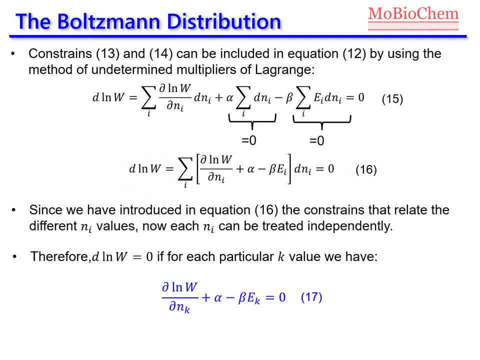 logarithm of w will be equal to 0 if each of the terms in this summation here is also equal to 0, so we can write then equation 17.. And now, in order to solve this equation, what we have to do first is to compute this derivative. 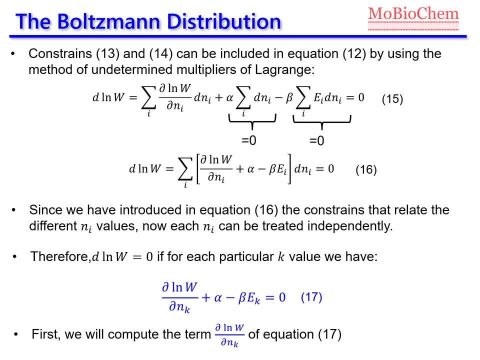 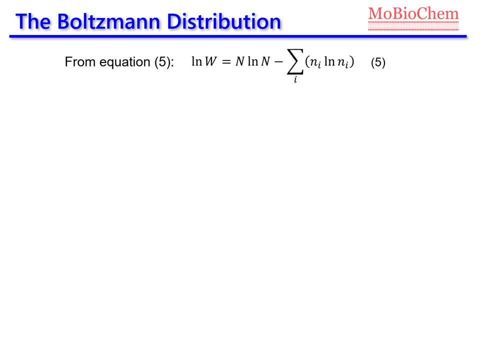 which is the the complicate part of the equation 17.. Okay, so, in order to compute this derivative, let's start from equation 5.. Equation 5, if you remember, provides the logarithm of the weight w after applying the Stirling approximation a few slides ago. 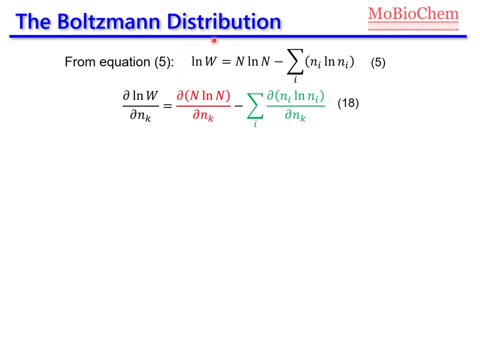 Okay, so let's do the derivative of this equation with respect to the number of molecules in the state k. so we have to do the derivative of each of these two terms. For the moment it is easy, And now we are going to solve these two. 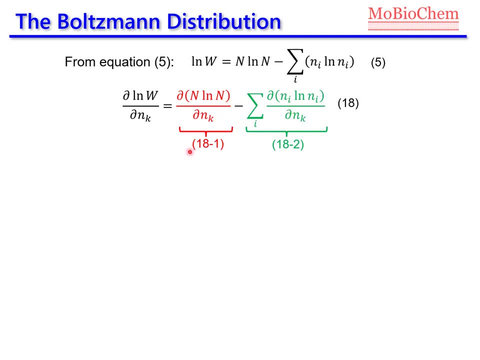 derivatives in an isolated way. So let's start by the first term, 18, 1.. So here we have the derivative of a product with respect to Nk. so this is derivative of the first term, N with respect to NK, multiplied by the second. 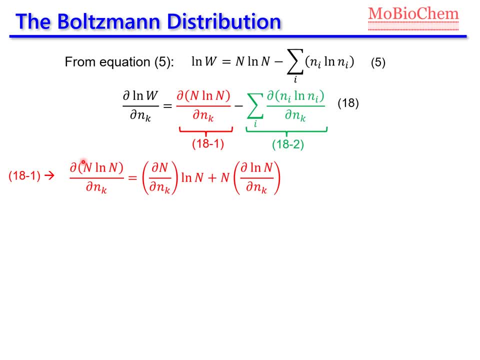 term as it is here, and now we have the first term, N, as it is multiplied by the derivative of the second term. okay, now the total number of molecules, capital N, is the number of molecules in the state number one plus the number of molecules in the state number two, and so on and so forth, and this is equal to one. 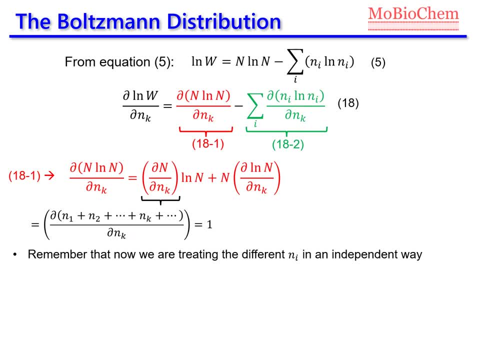 because the derivative of N1 with respect to NK is equal to zero. the derivative of N2 with respect to NK is also equal to zero. the only term which is not zero is the derivative of NK with respect to NK, which is equal to one. and remember that this equation is true because now we are treating the 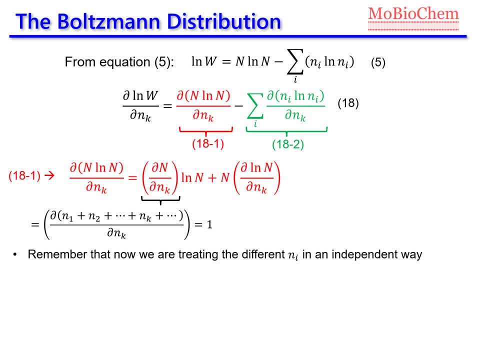 different populations in a independent- independent way, because otherwise, remember that the different populations depends on each other- and then this equation will be not equal to one. okay, but as we are treating the populations in an independent way now, we can apply this simplification at this step. okay, in this second term, we 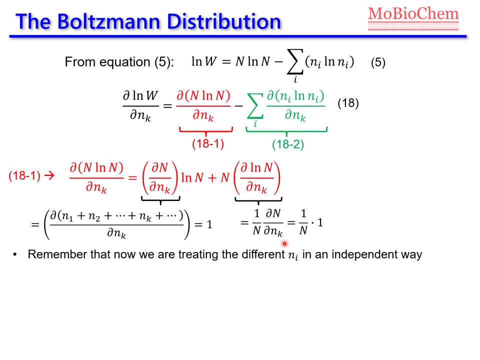 can write the derivative of the logarithm in this way and using the same reasoning. so this derivative of the total number of molecules with respect to the population of K is also equal to one. so it is the same situation as we had here before. okay, okay, so the term 18-1 can be. 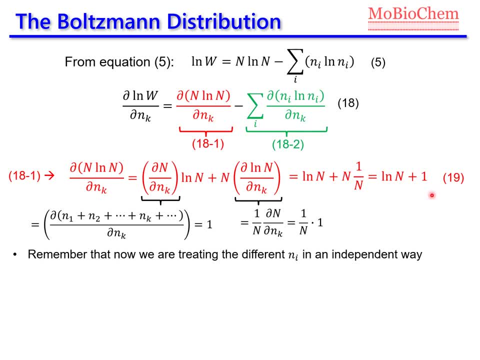 written as the logarithm of the total number of molecules plus one. after applying these simplifications, now let's have a look at the second term of equation 18.. so we have again the derivative of a product here. so this is the derivative of the first term multiplied by the second term, as it is plus the second term. sorry. 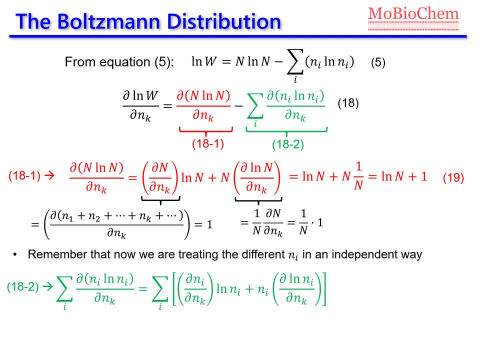 the first term as it is multiplied by the derivative of the second term. so this is easy and here this is remember. all of this is inside this summation here which runs over I, and here we have the derivative of the number of molecules in the state I over the derivative of the number of molecules in the state K. 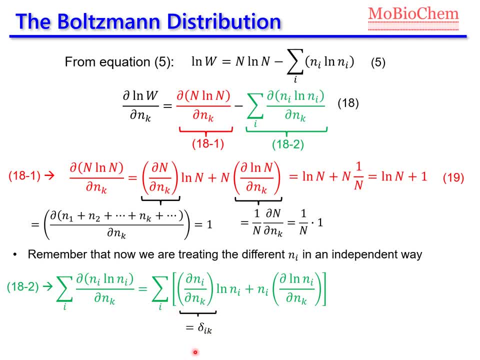 and this is equal to the delta chronicle, right, because this is equal to one only in the situation where I is equal to K, as we said before here. in this part of this equation, as we said here, all the other derivatives are equal to zero and what we have is the derivative of a product. it is called a derivative of a. 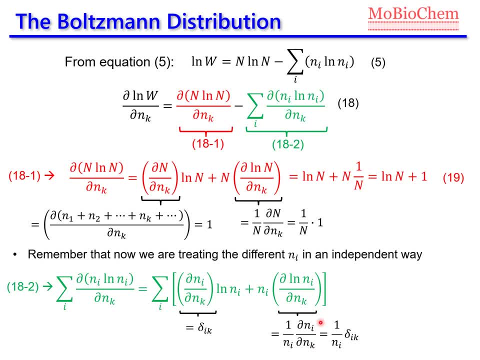 mnie over N. so now, if we were to make such a situation that the mannequin of this aufge can pass over to the other plugin, G, over the derivative of this對不起 here. now, this derivative- here is the derivative of I- is equal to K. so we have only here logarithm of NK and here the same thing. 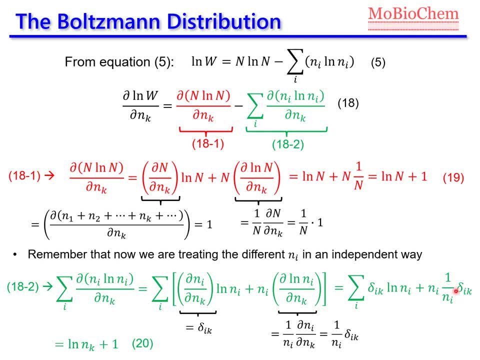 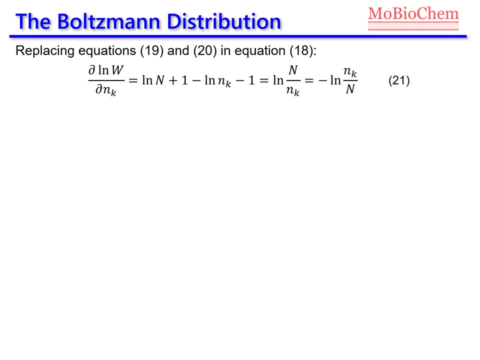 when I is equal to K, this is 1, and NK over NK will be also 1. therefore, we have here just 1. okay, let's replace equations 19 and 20 into equation 18, and we got equation 21, where the variation of the logarithm of 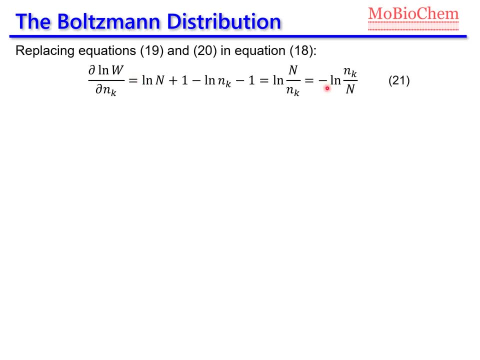 W with respect to the population of K is just minus the logarithm of the population of K over the total number of molecules. so now we are going to insert this equation into the equation 17th that, if you remember, equation 17th was this equation where we we said a few slides ago that we are going to solve. 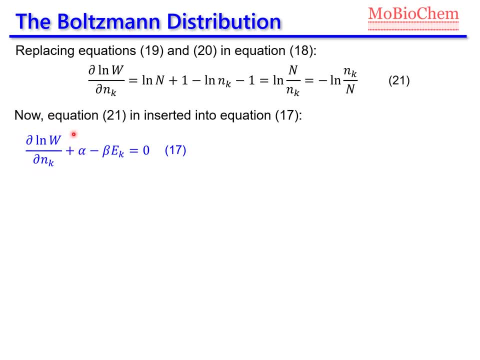 first the equation 17th. so we are going to solve it now, this first derivative which is the complicate part of the equation, and now we have here the solution of this derivative. so we replace this solution here in equation 17, and we got equation 22,. 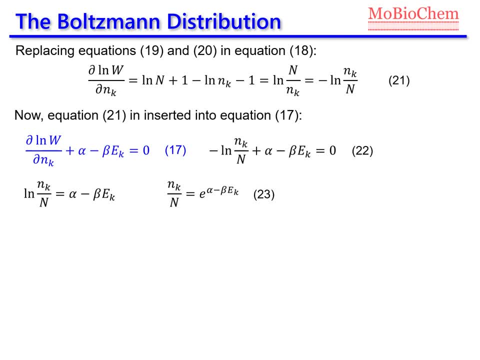 which can be rearranged in order to get equation 23.. Finally, we can isolate the number of molecules in the state number in the state k, sorry, and we got equation 24.. Okay, we are going to keep this equation for a minute. 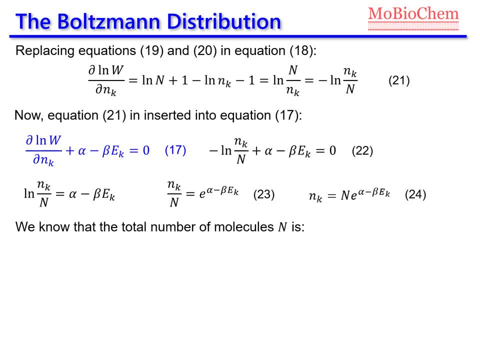 and now we know that the total number of molecules n is just the summation of the molecules in every state k. and now we replace equation 24 here and we got this equation where we have the exponential of this difference here, which can be written as the product of these two exponentials, right, And now the total number of molecules- n is just the summation of the molecules in every state k. and now we replace equation 24 here and we got this equation where we have the exponential of this difference here, which can be written as the product of these two exponentials, right, And now the total number of molecules- n is just the summation of the molecules in every state k. and now we replace equation 24 here and we got this equation where we have the exponential of this difference here, which can be written as the product of these two exponentials, right, 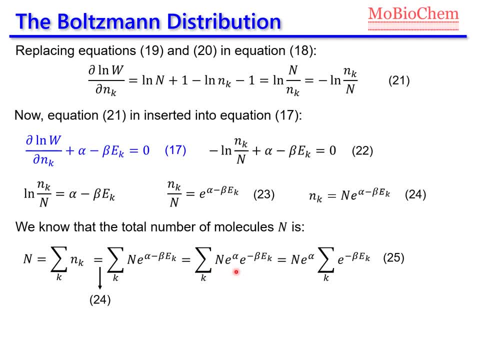 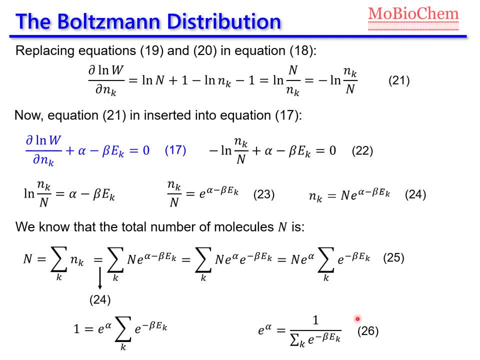 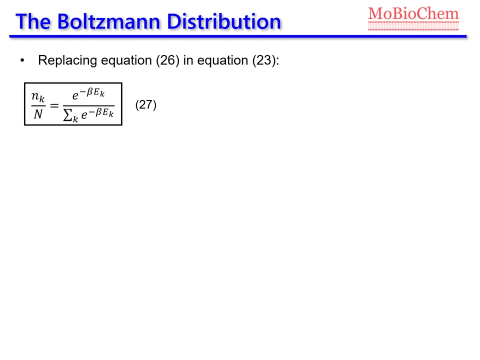 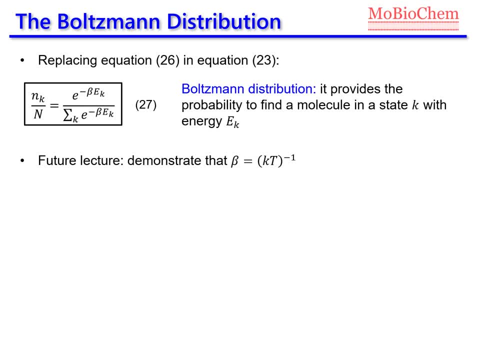 in a state k with energy ek. In a future lecture we are going to demonstrate that beta in this equation is the inverse of the Boltzmann constant multiplied by the temperature, but we are going to talk about this in a future lecture. If you look at equation 27,, you can see that the distribution 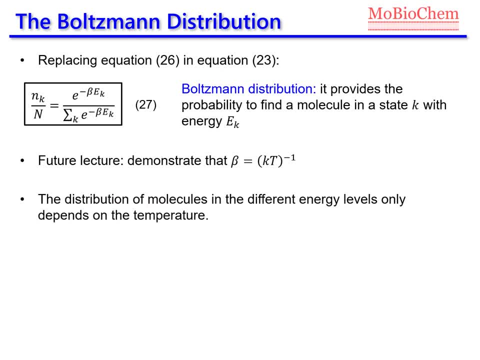 of molecules in the different energy levels depends only on the temperature. This is one of the conclusions of the Boltzmann distribution. In addition, the Boltzmann distribution depends here, in the denominator, on what is called the molecular partition function, which provides an estimation of the number of states that are accessible to a given temperature. However, 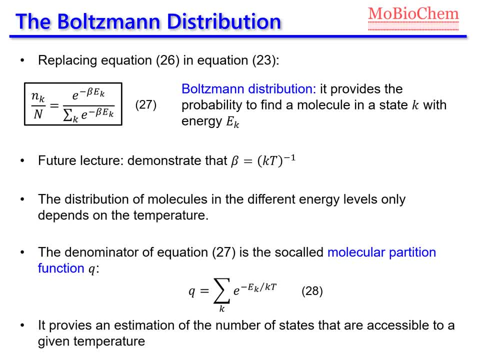 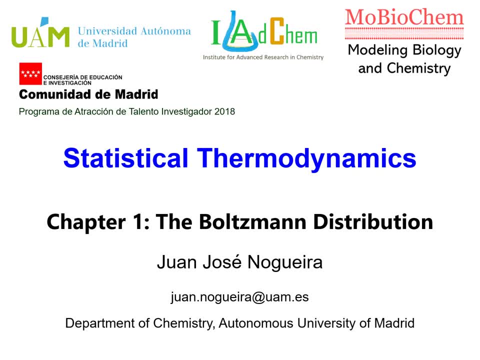 we are going to talk about the partition function also in a future lecture. That's it. Thank you very much for watching and see you in the next lecture. Transcription by CastingWords.